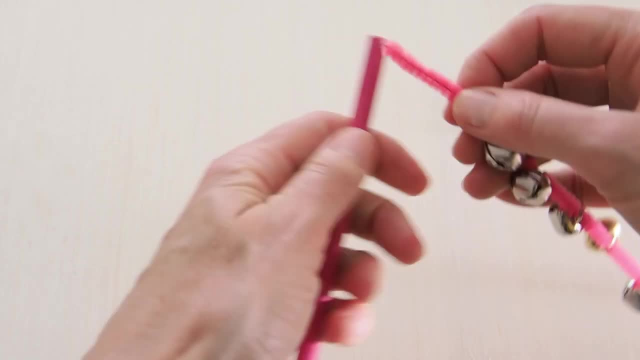 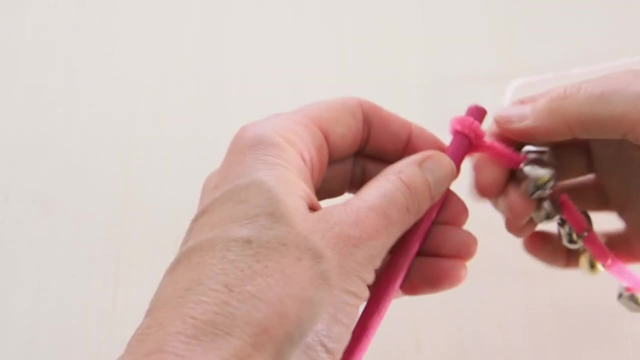 jingle bells on your pipe cleaner. you're going to twist the pipe cleaner around the top of the pipe Stick that you have. we're going to twist that really tight. we don't want it sliding off the top. you don't want it too close to the top or it could slide off. and we've left enough room so that we can. 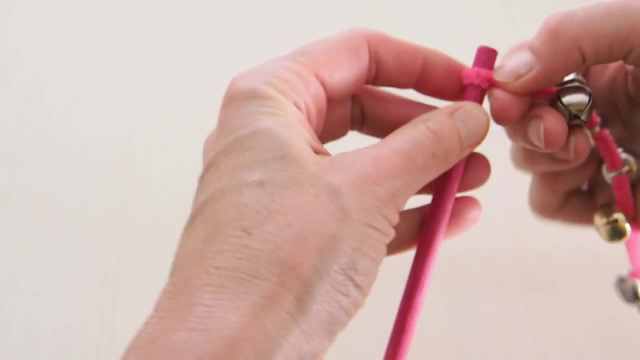 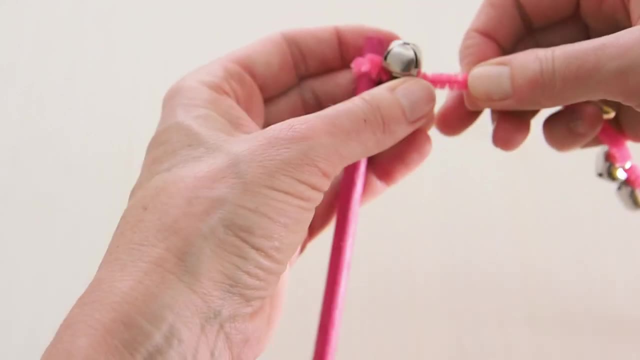 easily do that. Again, we will rearrange our jingle bells as we're twisting it down the stick so we'll get the spacing right on those as we go along. So then you're simply going to push your jingle bells where you would like them and start twisting your pipe cleaner around the stick, just spacing those. 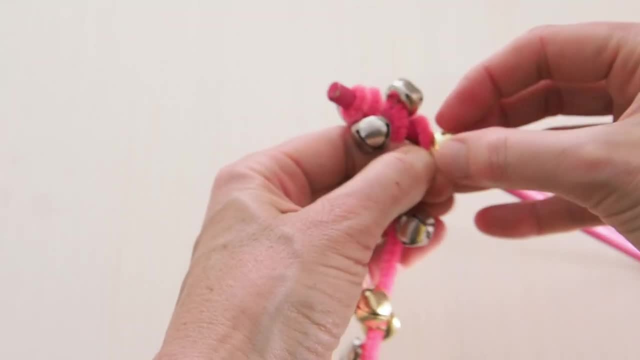 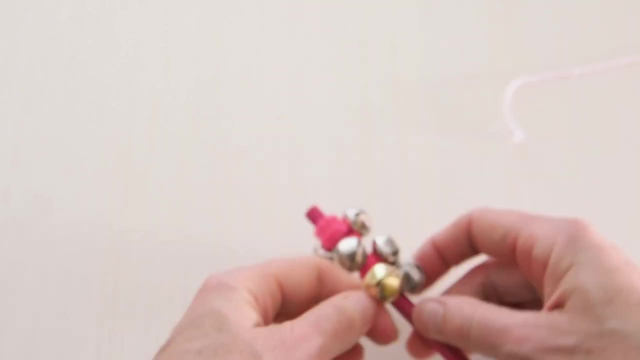 jingle bells as you go. There's no right or wrong to this. however you do the spacing, I just kind of twist as I go. if I see an empty space that looks like it needs filling with a bell, I just twist one in there and fill that spot in. So keep twisting all the way. 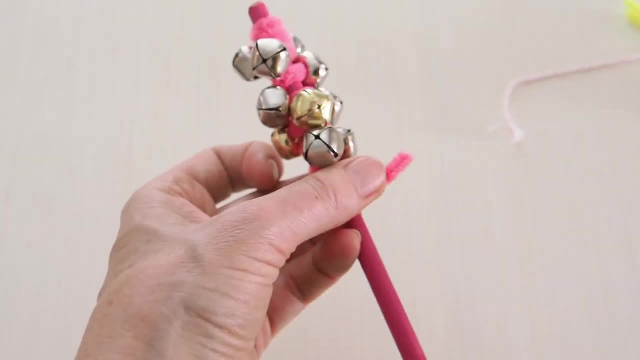 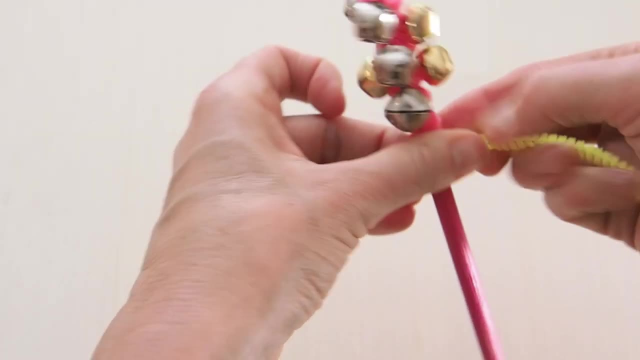 down to the bottom of your pipe cleaner, So you'll be about a third of the way down the stick when you're done, and then you'll get another pipe cleaner, Stick it back up so we attach it tightly to the other pipe cleaner and then we twist in the opposite direction. 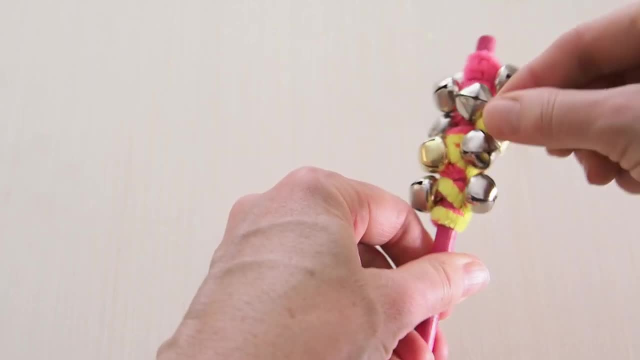 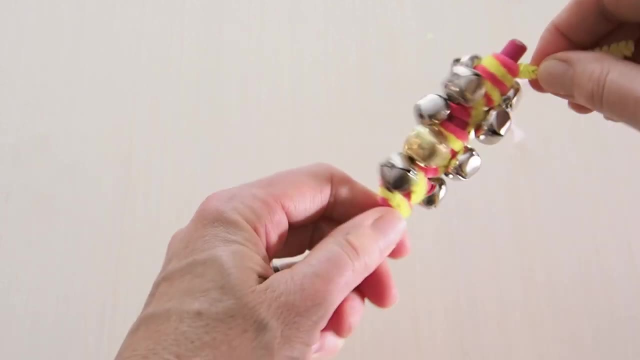 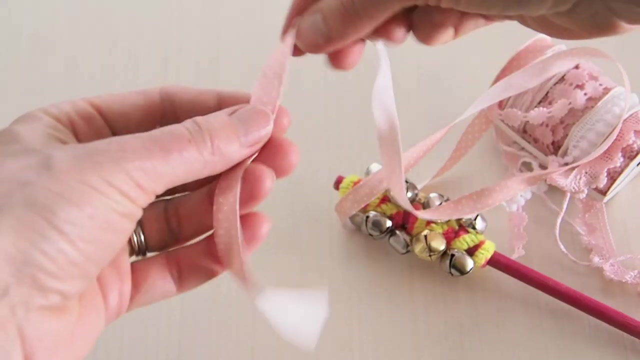 We're going up through weaving in and out around the bells and we get to the top and we're going to twist it around tightly at the top and now we'll start to tuck it in a little bit and then get our ribbon. So I cut generally just a couple inches of ribbon. that's up to you. I think I used about a. 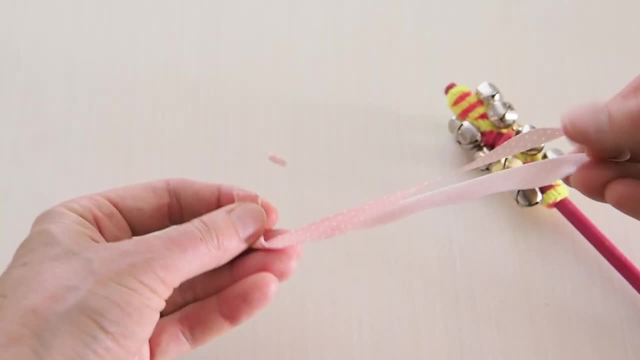 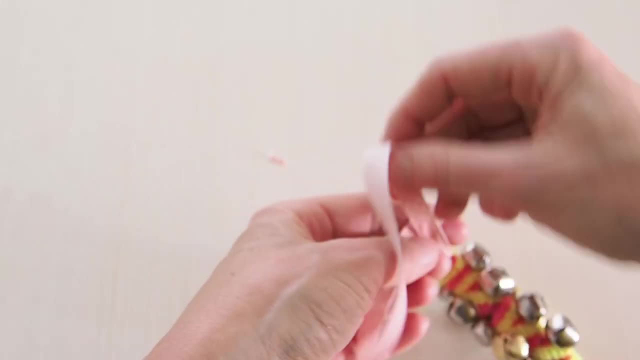 four inch, well, a total of eight inches of ribbon. so there's four to five inches side And then we just put the loop through the pipe cleaner, knot it onto the pipe cleaner so it stays really well. Then we're going to twist the pipe. 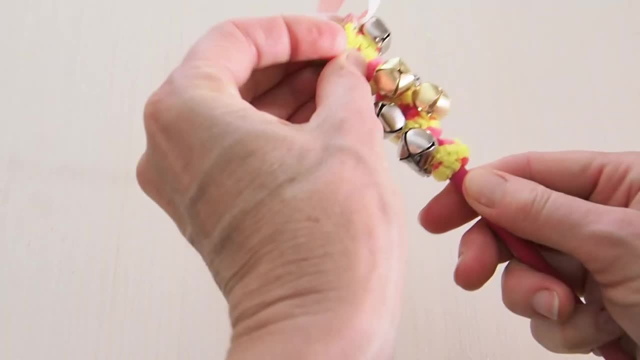 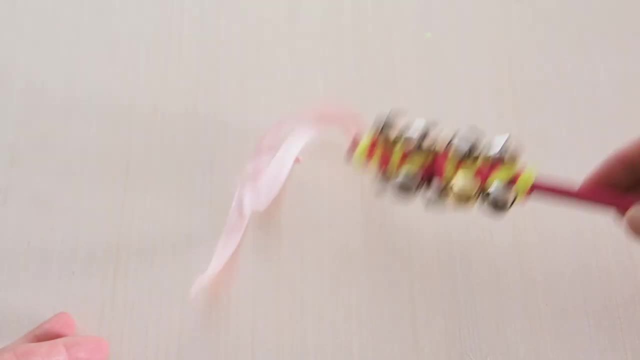 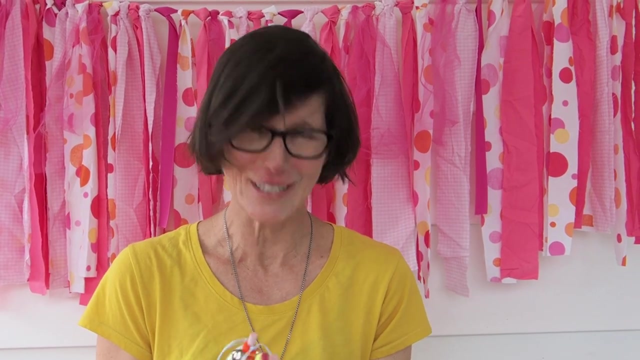 cleaner onto the stick and tuck the end of it down underneath the bell, because we don't want that sharp point of the pipe cleaner sticking out. So I hope you enjoyed making these as much as I did. They just always turn out so cute It's like I have to jingle them If you have any comments or if you.